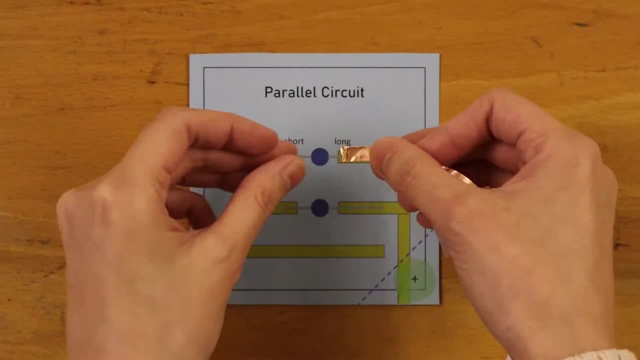 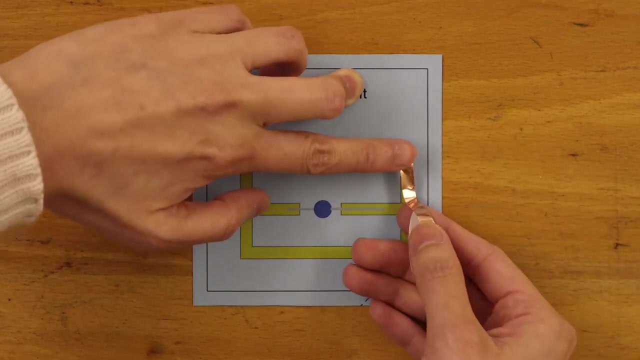 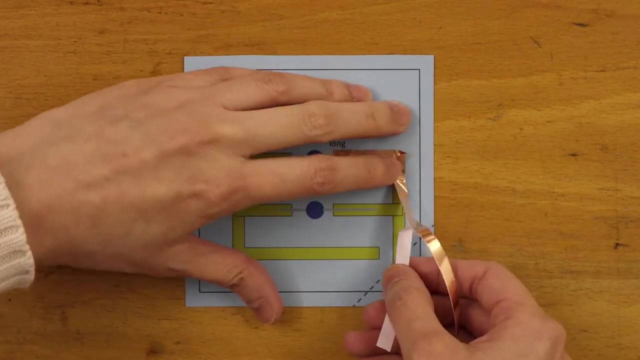 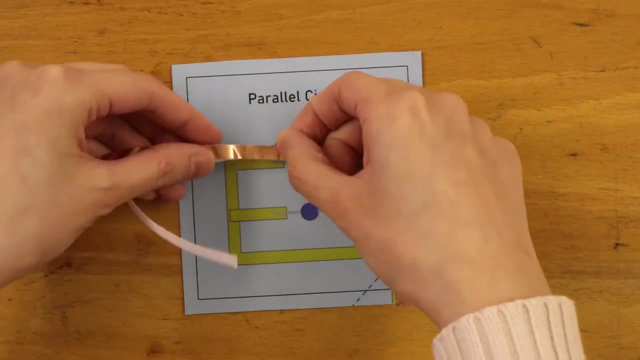 When turning the tape around a corner, be sure not to tear it. Try to fold it down so that we can keep the tape continuous. Do the same on the left-hand side. If you do happen to tear the tape, just make sure that you continue the cutting. 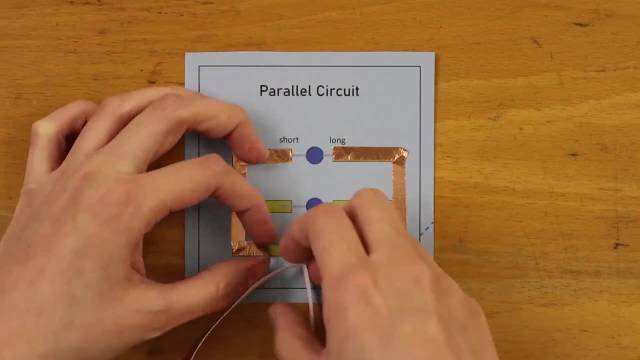 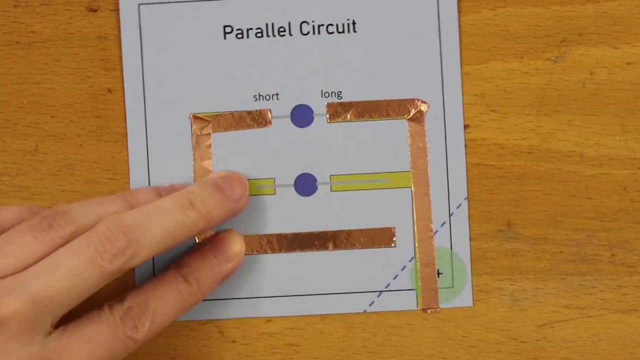 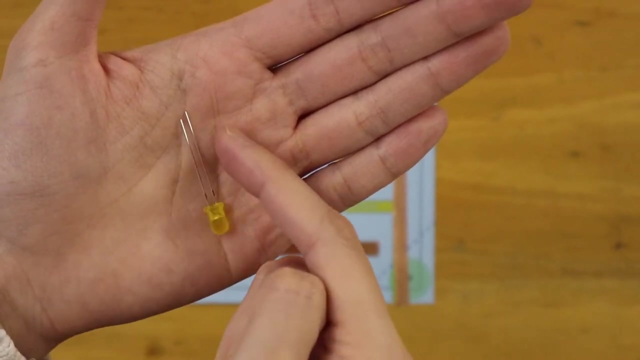 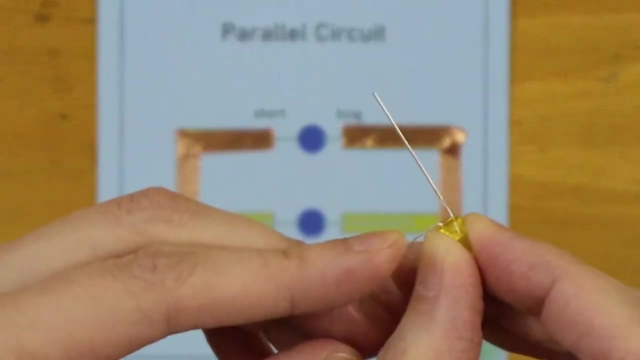 You can also remove the copper tape by overlapping where you've torn it off, And here I am making sure that the copper tape is nice and flat. An LED has a long leg and a short leg. The longer leg is the positive side and the shorter leg is the negative side. 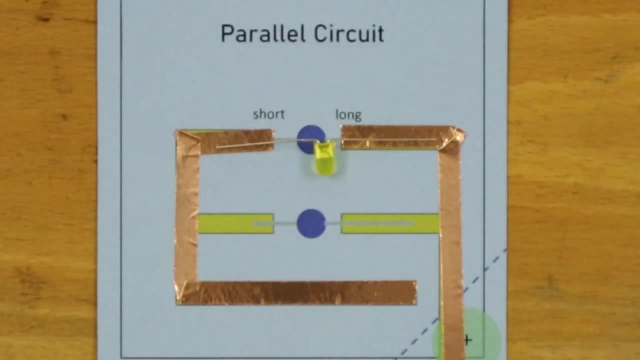 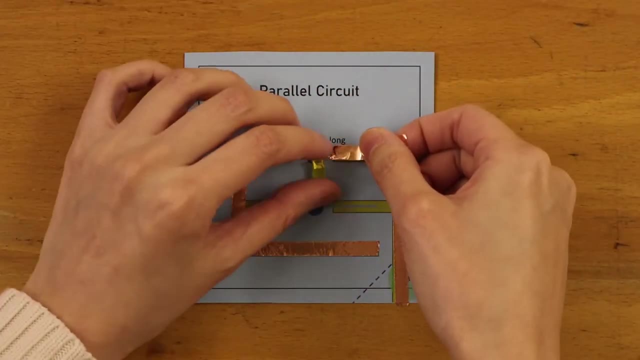 The positive side of the LED connects to the negative side. The positive side of the LED connects to the positive terminal of the battery. Let's secure the connection of my LED to the circuits by using more copper tape, sticking it over the legs of the LED. 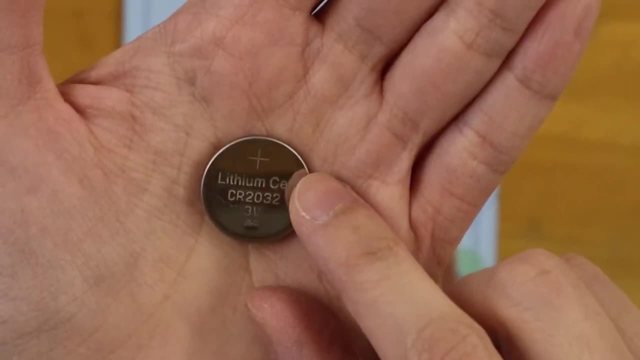 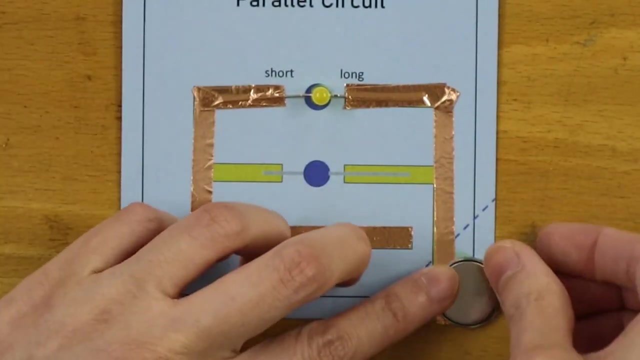 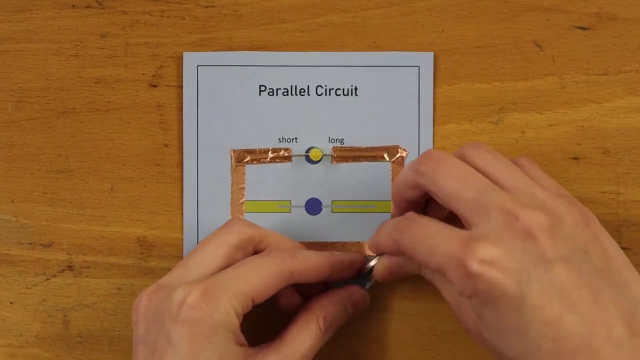 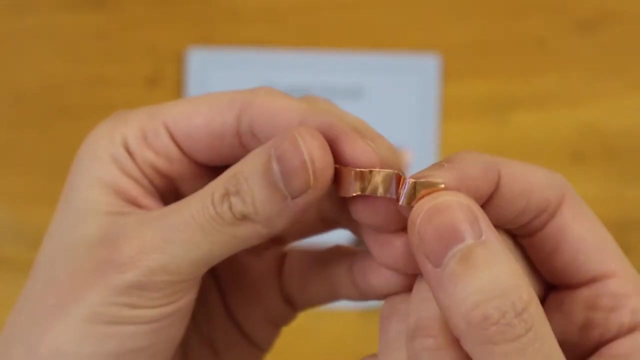 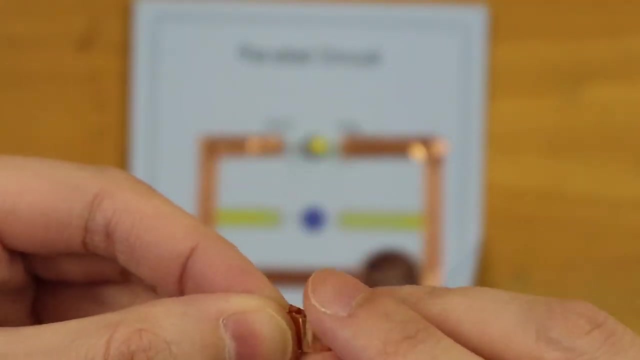 The bottom side of my coin battery is the positive terminal. I want this facing down on the coin. It's very hard, Once I'm sure the circuit is working properly, stick the battery in place. To do this loop a small piece of copper tape with the sticky side facing outwards. 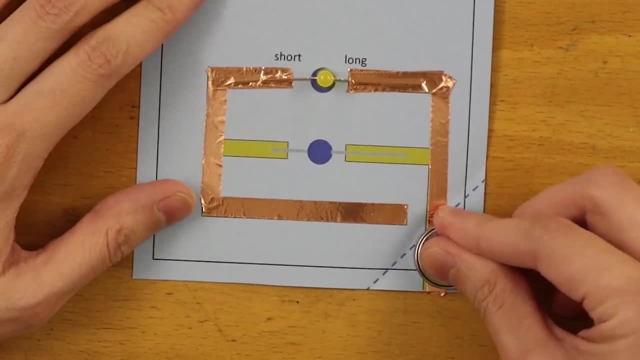 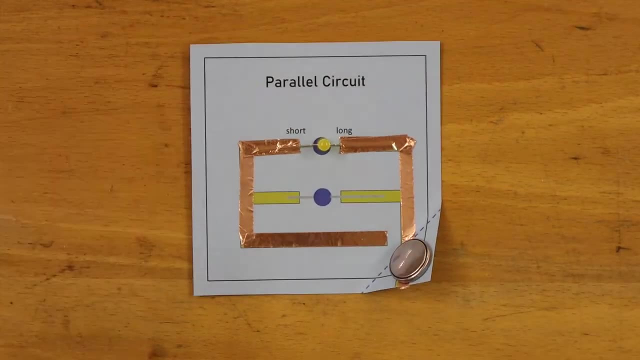 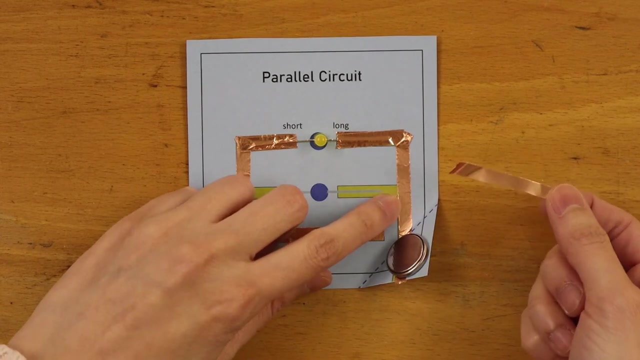 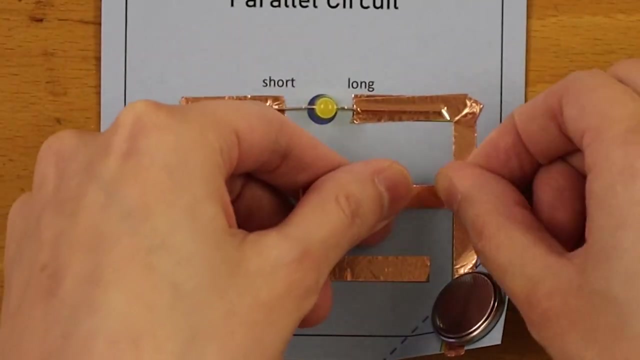 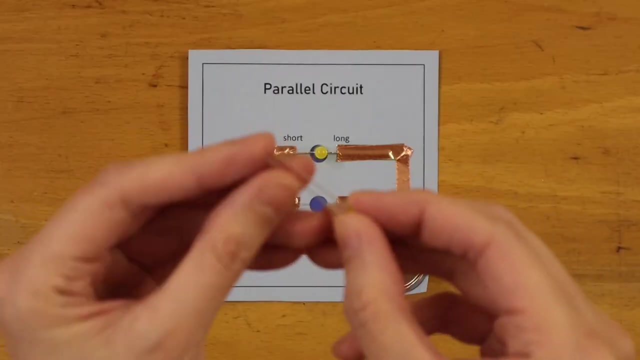 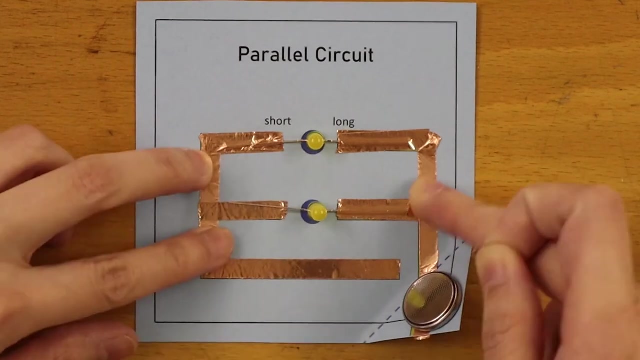 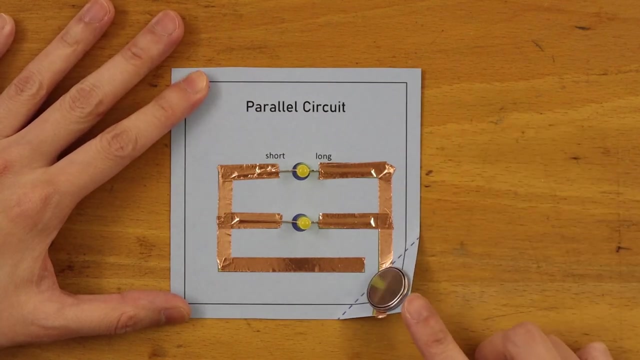 Right now I just have one loop and I want to turn it into a parallel circuit. When making this new branch in my paper circuit, remember to overlap the copper tape with the outer loop. And now the moment of truth. Thanks for watching. Be sure to subscribe for more physics.